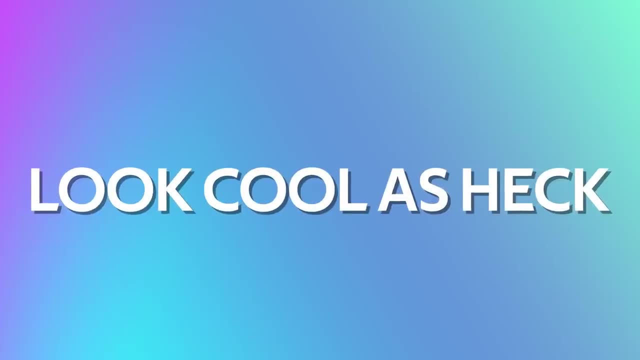 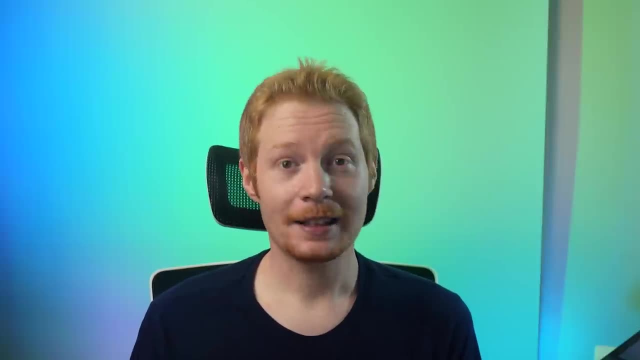 readability at a glance, while containing a ton of information, and still look cool as heck. So how do you do that? In this video, I'll show you how to design a card from scratch explaining the reasons behind each decision, the best practices and why you must obey these five. 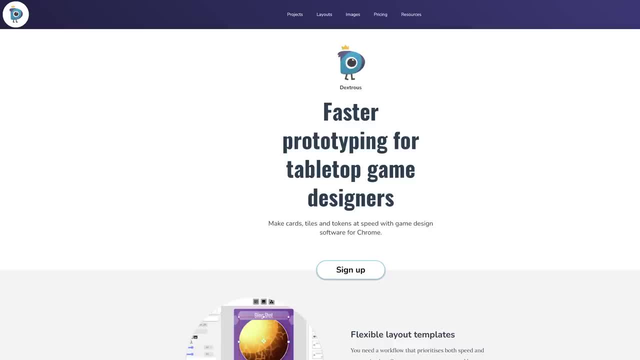 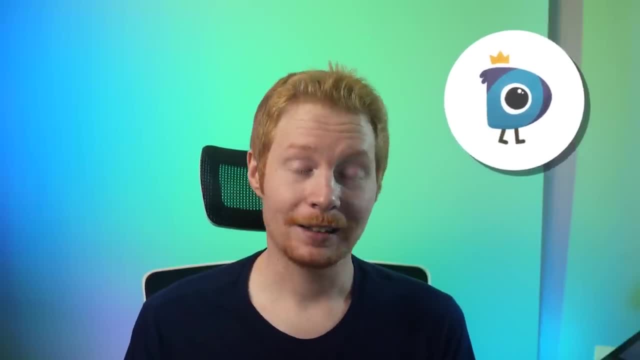 golden rules, And I'm going to do that on the Dextrous website because it is free and easy to use, But more importantly because it allows you to make sweeping changes to every card in your game at once, And that is legitimately a game changer when making your game. More on that. 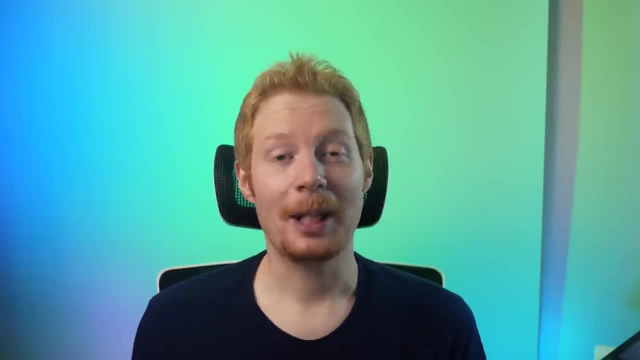 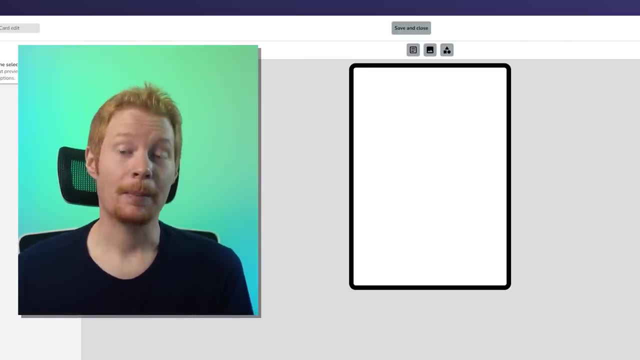 later. Hi, my name is Dave Jeltema. Welcome to Tabletop Craft. Let's get started. First things first. I am starting with a blank poker size card, since that is by far the most popular option. But don't worry, all the information in this video is still relevant to any card you want to design. 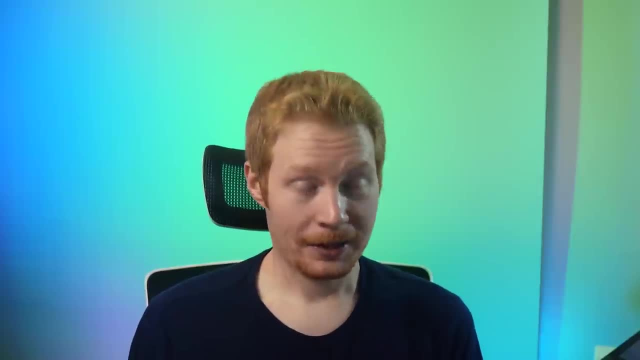 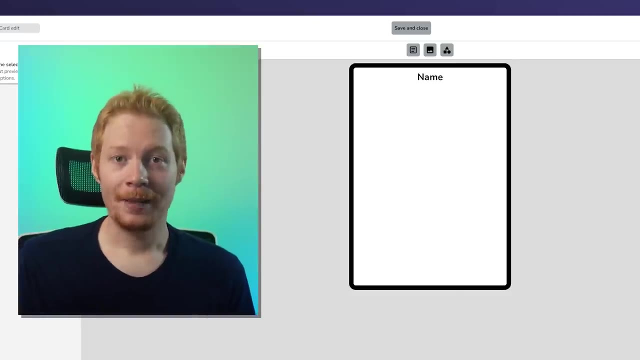 Whether it's horizontal mini tarot, it all applies, And so the first question to answer is: what all goes on a card? What information is important for your game? It'll probably need a name and an effect and some art, But let's make a few more assumptions so you're better equipped. 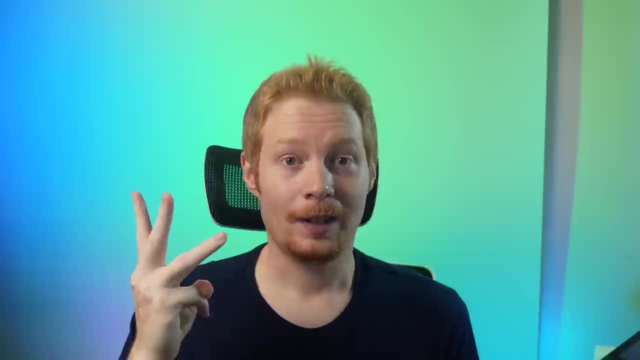 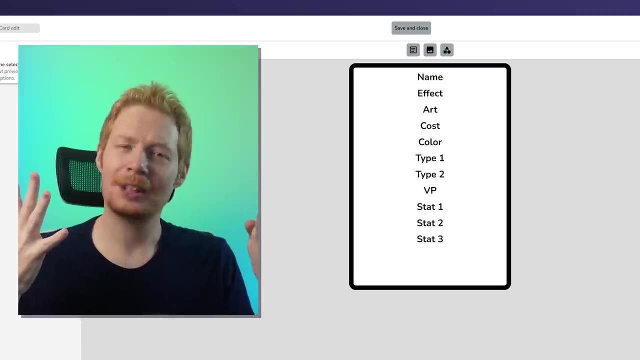 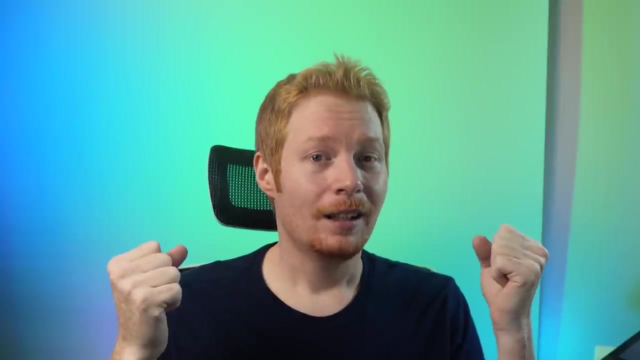 to design your own card. I'll use our game as an example. Our cards also have a cost, color, two different types, a VP value and stats that we might soon change to dice. That's 9 to 11 different things. to fit on a poker card Doesn't sound too bad, But when you want the card to look, 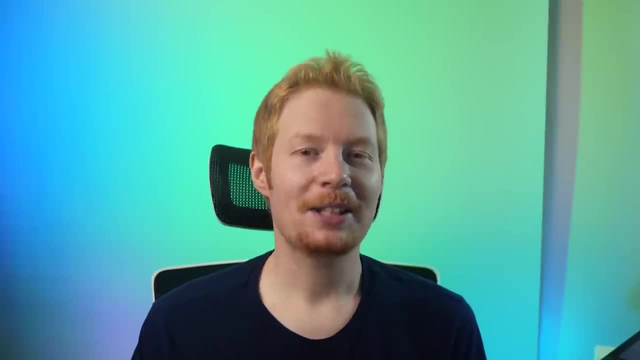 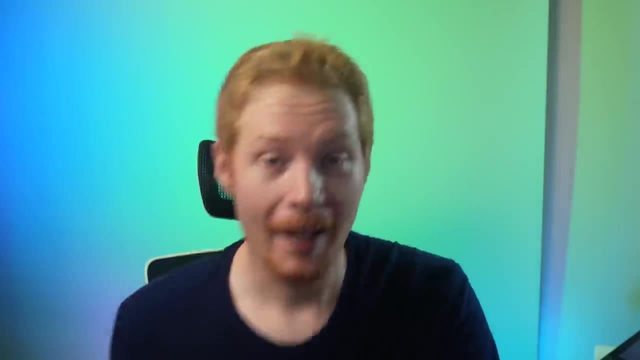 good and the information to be reasonable. you can use a card that has a lot of value. I'm going to get this blank card set up with all the elements I just mentioned, But, as I do, I want to show you something and then ask you a question. I have had this hanging on my wall. 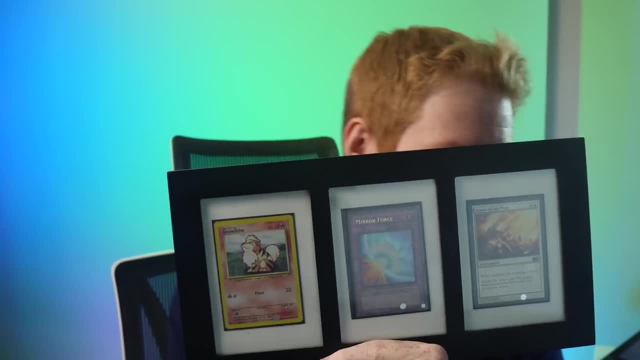 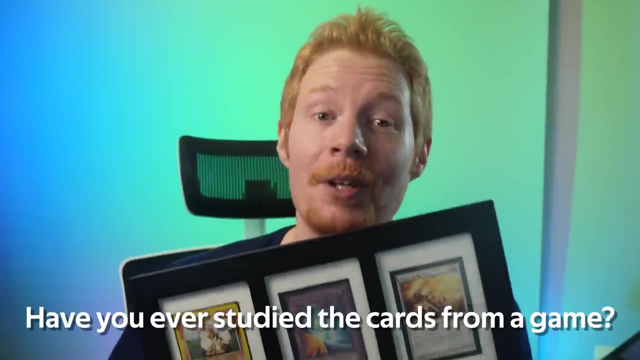 for a few years now. It is a tribute to my three major CCG addictions. We have elementary, middle school and high school. My question is: have you ever studied the cards from a game? Ask yourself why the cards are laid out the way they are. Each of these follows a. 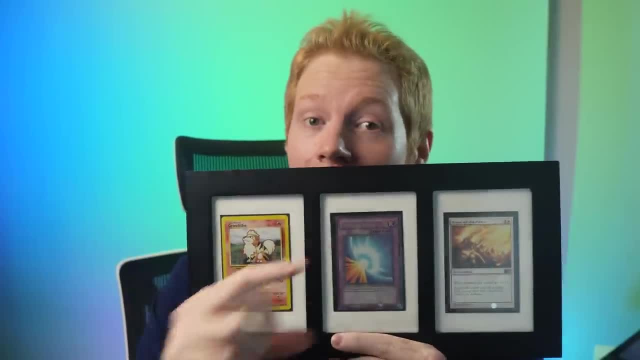 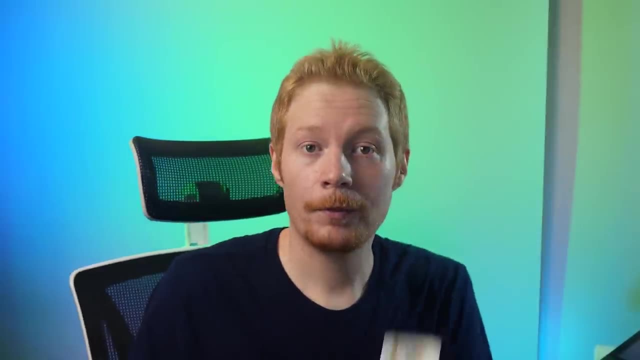 similar format. You'll notice that the titles are above the effect and that the art takes up more space than any other element. Let's look at a more current example. This is a card from Farshore. It is a game that was released at this year's Gen Con. You'll notice some similarities. 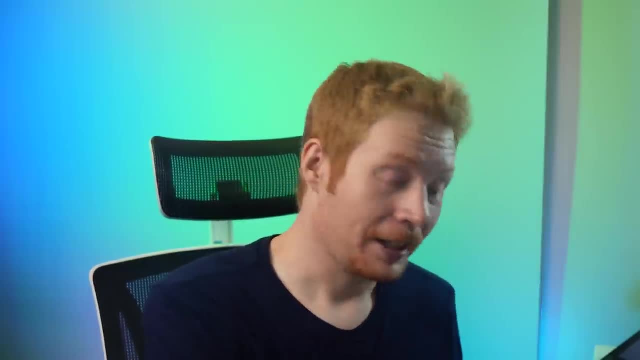 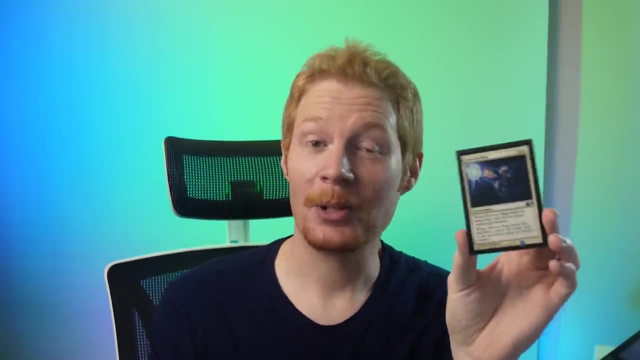 but the key difference is in the top right corner. Let's single out Magic. the Gathering Its cards are a prime example of breaking the first golden rule. It is well known for breaking what has become conventional wisdom at this point because its cards were designed before. 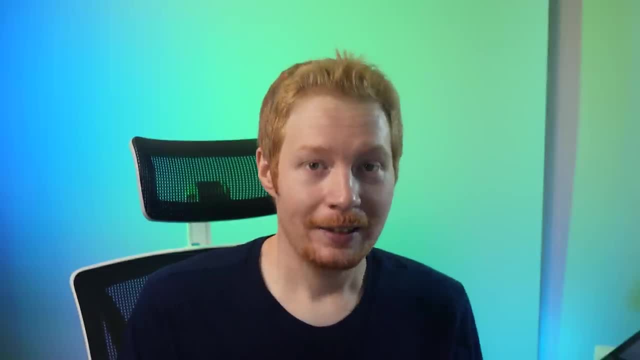 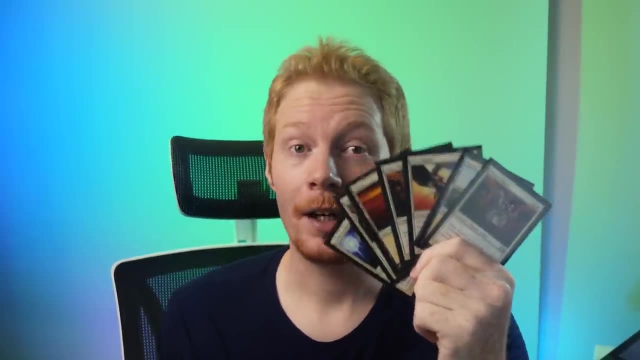 it became conventional wisdom. It is a card that has been used for a long time and it has been used for a long time. To explain this, here is a hand of cards that you might typically see when playing. Most information, the most important information to compare among cards at a glance. 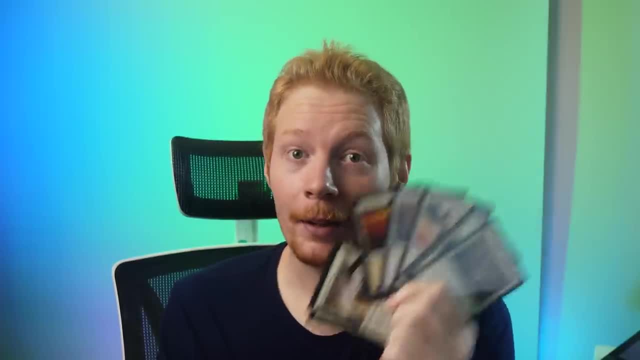 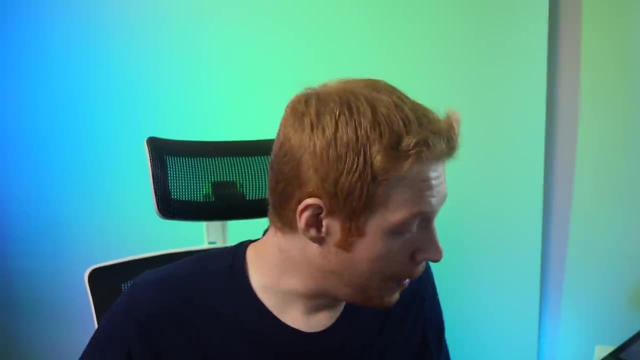 is their cost, which is completely hidden when fanned out in your hand. When designing your cards, consider what might get covered up. But cards in the hand aren't the only way that things can get covered up. Here are a few example cards from our game. Ignore that one I forgot to tell. 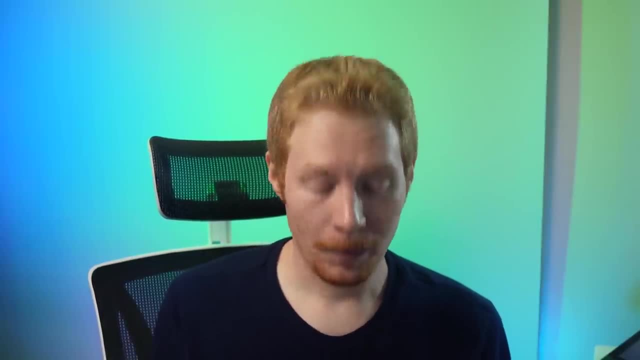 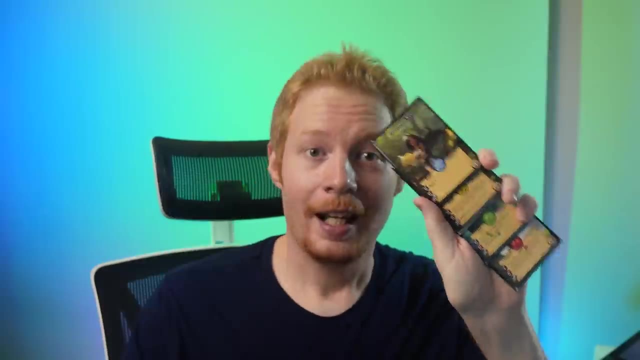 them the right size of paper. Whoops, We have a mechanic in our game where you can stack stack cards to repeatedly get their effect. By placing this one on top, it activates everything in the chain until the new card activates. We need to be mindful that the types remain visible. 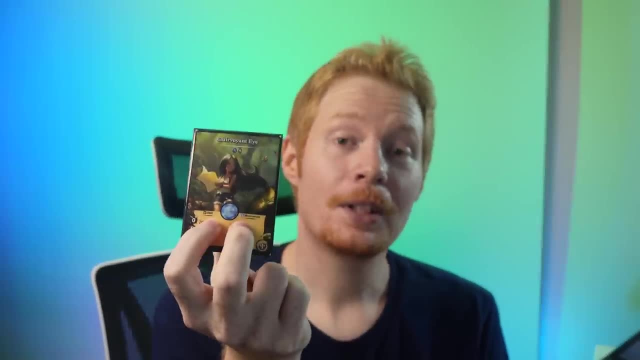 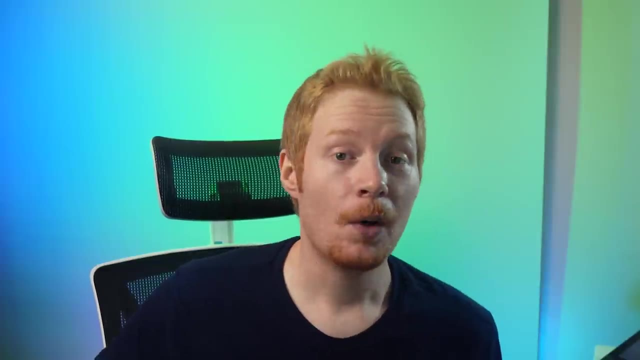 because other cards reference them. It is important to know how many of which types you have, whereas the cost can be covered up because it's only relevant to our game when purchasing the card, If we ever considered a mechanic that looked at the cost of a previously purchased card. 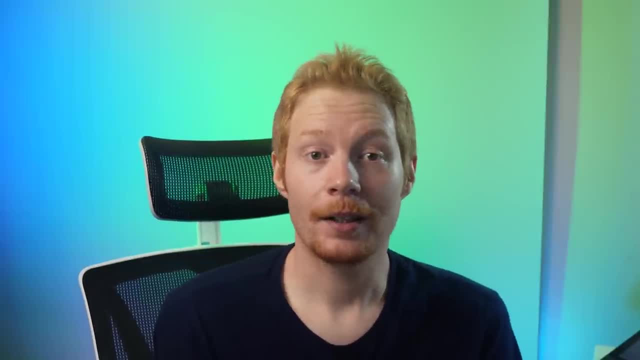 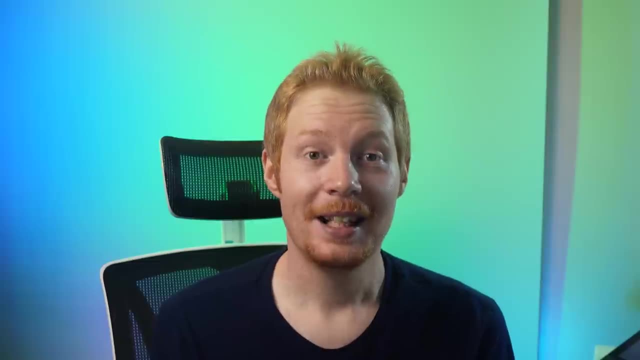 then we could have a problem because this mechanic covers up some of those cards. So golden rule number one is to never obscure vital elements. Don't think you can get away with it, because magic does. They are the exception to the rule because time And here we are, back to our less blank card and we learned 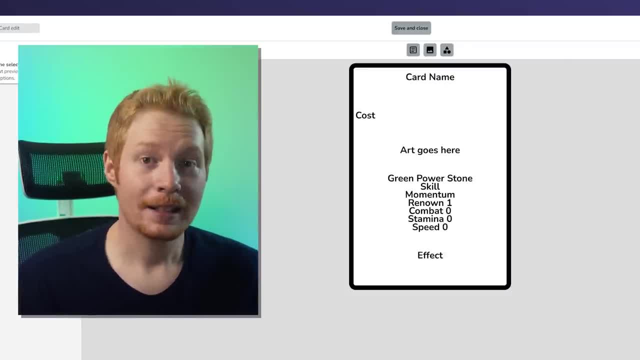 that we like the cost over here on the left and we saw that it makes sense to have the name of the card at the top or maybe the middle, so long as it's above the effect text And we know that we could maybe hide the VP, but I like the idea of using it as a way to gauge the effect text. 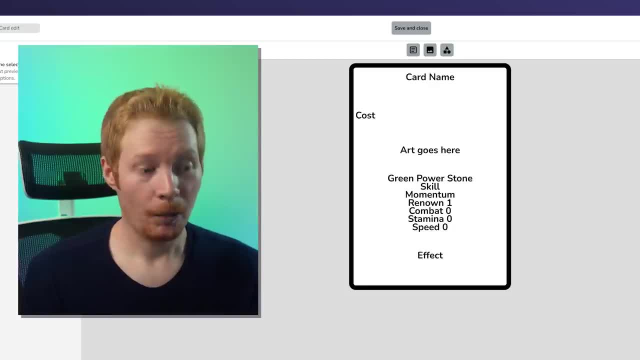 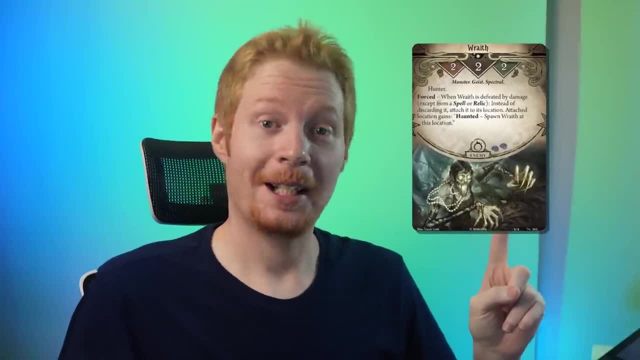 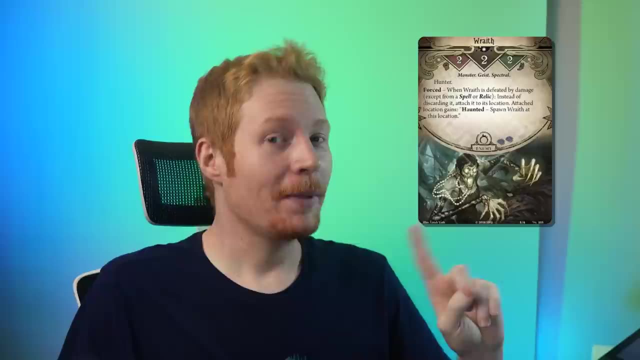 But what about everything else That leads us to the next golden rule? Here is an example card that follows the second golden rule. I stole this example from Matt Paquette from a blog post of his from five years ago. I like this card because it is something that 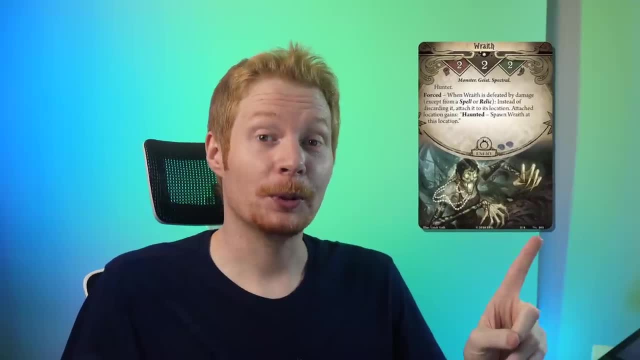 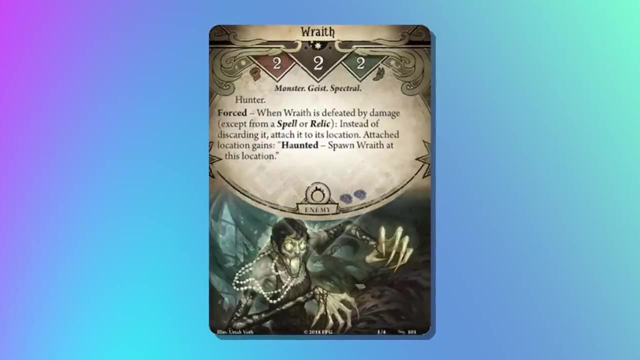 I would consider non-standard, but still exemplifies golden rule number two: What information is most important to your players? When I look at this monster card from Arkham Horror, the card game, the information is presented in a way that flows. My eye starts at the top with the name and the three numbers. Next the bold text. 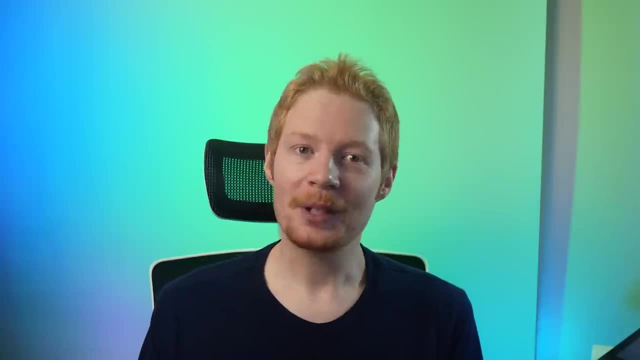 catches my eye and finally the text in the center. But then I realize I almost missed the three small icons in the card type underneath that text. Each of these elements is presented in a specific order, from most important to least, by its position on the card and the size of the element. 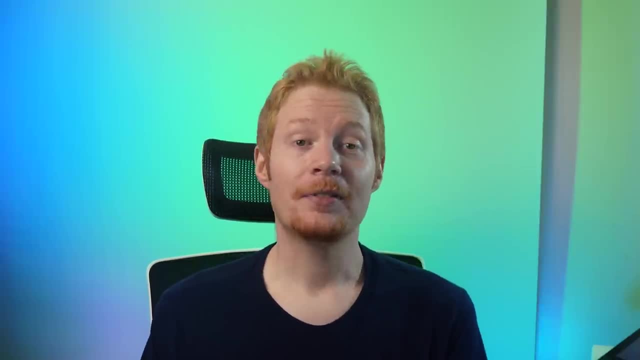 Imagine your card as the main branch of a family tree and then you divide it down into smaller sections or layers. The card's name and image should be at the top level because it is the most important information, but it's not the only one to be displayed: The card's name and image. 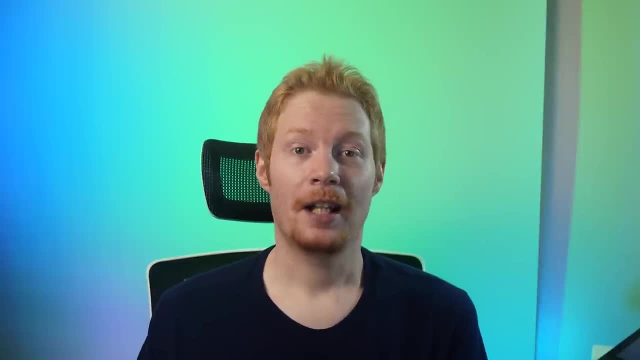 needs to be immediately noticeable, but then you move down the branch and move down the hierarchy, placing the less crucial details in order of importance and relevance. Things like flavor text will end up at the bottom. You can also think of this like telling a story. 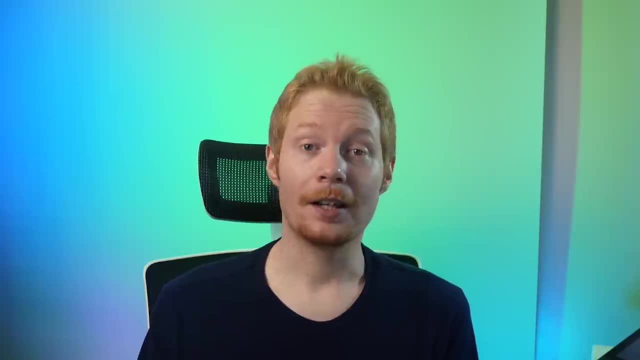 The main storyline is at the top, and if your players want to dig deeper into the card's detail, they can explore the sub-stories below. This way, players can quickly grasp the card's main purpose, while having the option to delve into more specific information if they want. 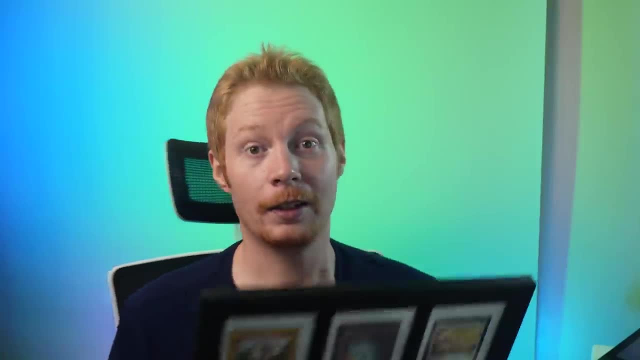 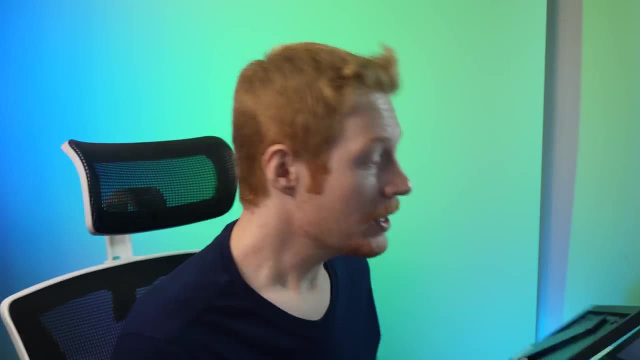 Let's go back to my framed example of the Yu-Gi-Oh card. This text is way too tiny for most games. They get away with it again because time, but also because the cards in your deck are something that you specifically understood. 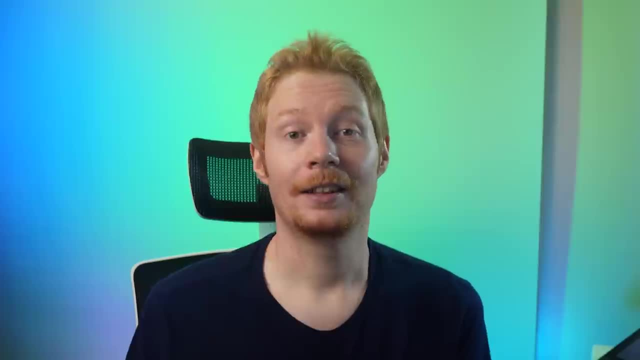 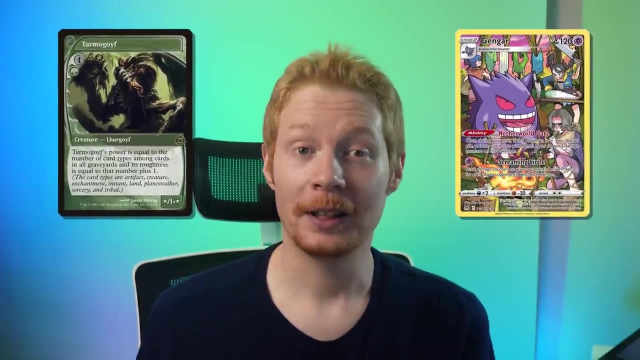 ahead of time and chose to be in there. and then they rest in your hand. But just look at all that wasted space. This card could look so much nicer. Magic and Pokémon have tried to iterate over the years, but people hate change. Everdell is a great example. I've played this game at least a couple of times and it's a great example. I've played this game at least a couple of times and it's a great example. I've played this game at least a couple of times. 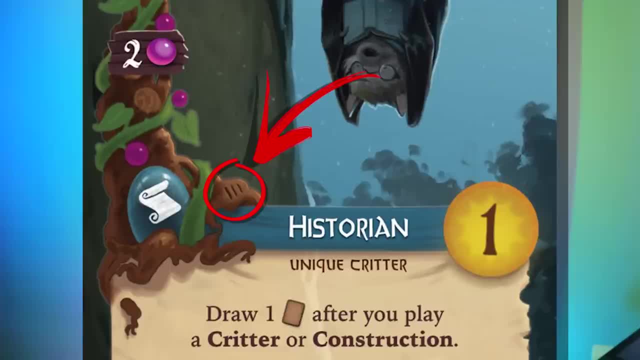 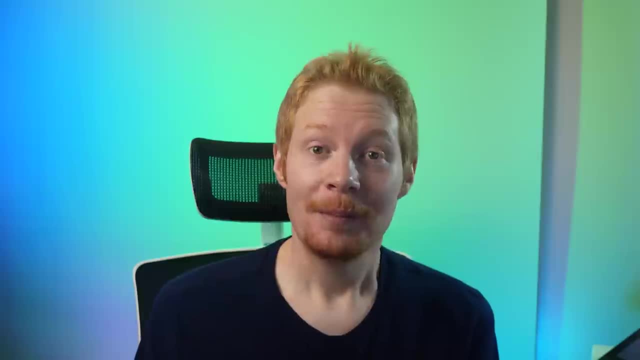 a dozen times at this point and until just recently I hadn't noticed these little notches in the wood on each card. Turns out they represent how many copies of the card are in the game. That's pretty cool, but very much not something that you'd want to put prominently. 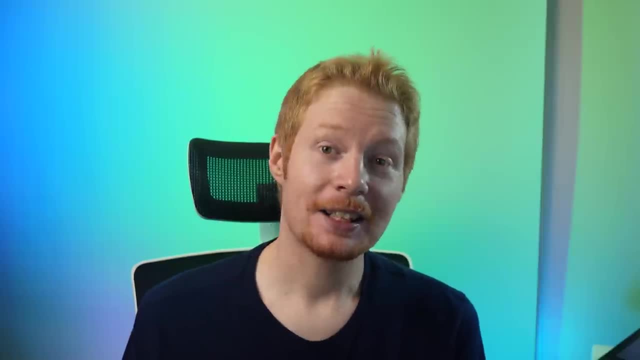 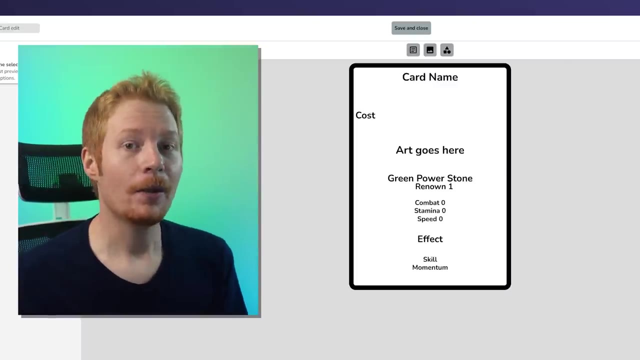 on the card, which is why this is basically hidden. Everdell is a great example of golden rule number two: follow visual hierarchy. So that brings us back to our card example. We know that the most important or primary elements are typically placed at the top. 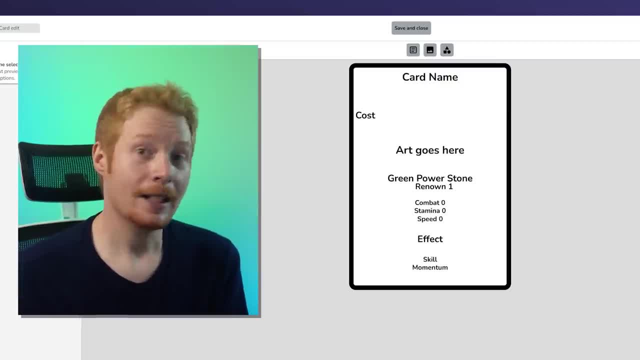 or forefront, making them more prominent and easily accessible, while less important or secondary elements are placed in the lower levels or layers. So that's why I've changed some of these to be bigger and others smaller, and I've reordered them by importance. The next step is to experiment a little bit. 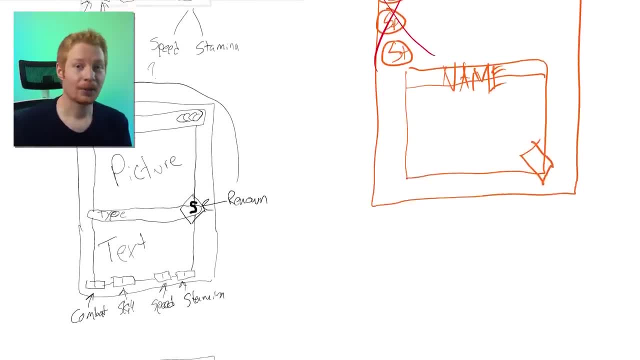 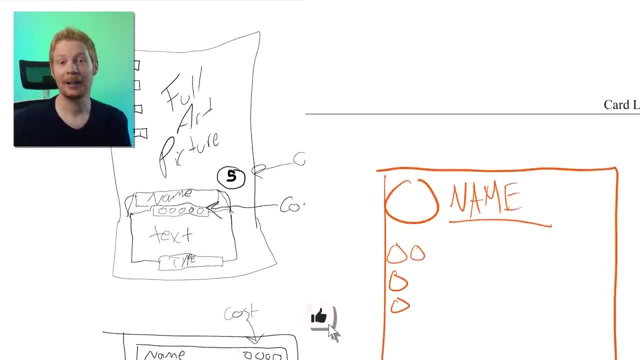 or a lot of it. Here you can see some of our quick and dirty sketches for our potential card layouts from our latest round of iteration. And just real quick, I want to take a second to ask you to take a moment and press the like button. It is my dream to keep providing you. 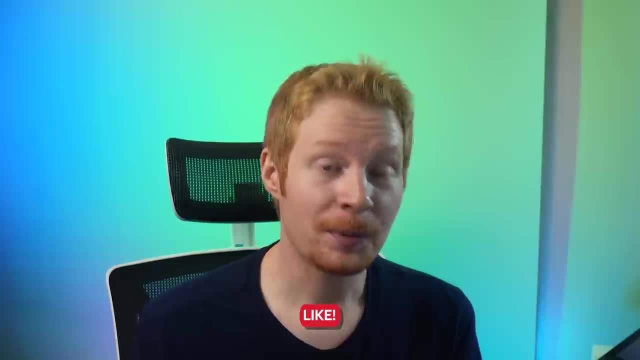 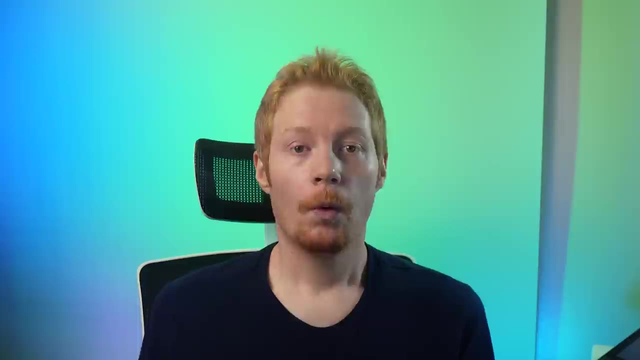 the best value I can, and you taking the time to press that button helps me grow and further define my content. Thanks for helping my dream come true. Okay, on to rules three, four and five. What makes a card readable? I touched upon it with the Yu-Gi-Oh card. Font size, spacing. 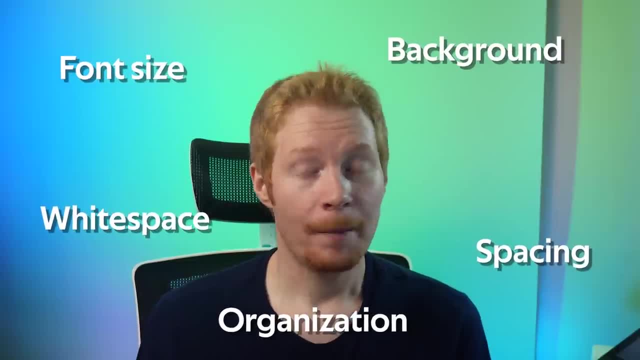 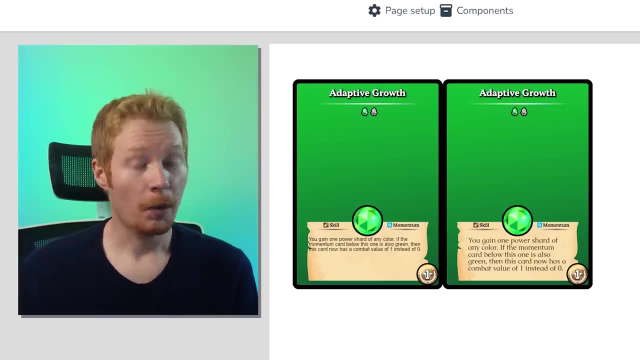 background: white space organization. All these are important factors, but they're all encompassed by the same idea. Here we have a couple of card examples I've mocked up. They both convey the same information. One of them is much more readable. On the left you can see the space between the border. 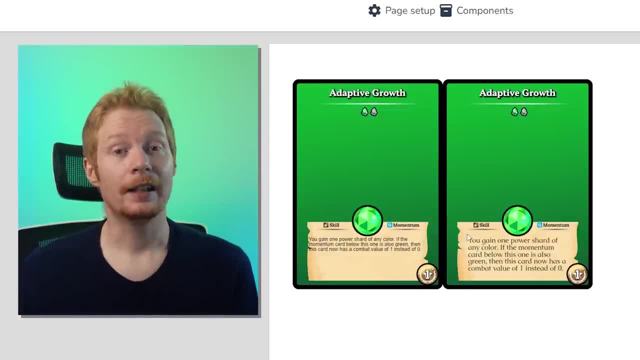 and the text could be a little wider. the font on the right is slightly easier to read and the extra between lines helps. Also, having font at eight points is a deal breaker for our game, because our cards are meant to sit on the table between all the players. Keep it simple and leave room. 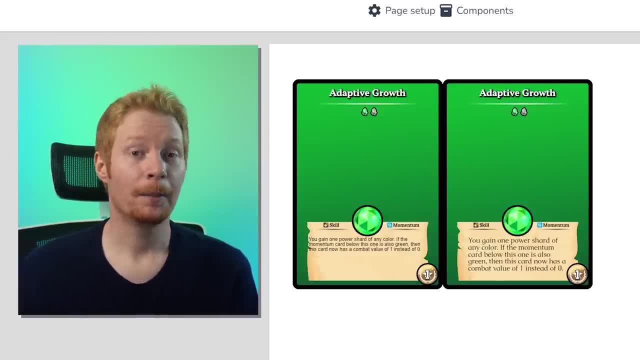 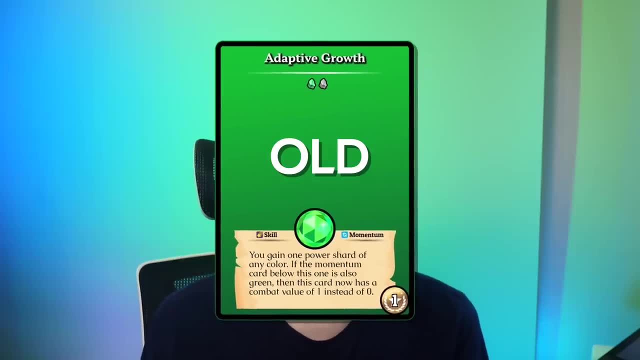 where you can. Your font matters and consider how far away the card will be read from. But the true golden rule to follow for readability isn't these things. If I take the card on the right, the better of the two, and apply golden rule number three to it, we get this instead and suddenly it becomes: 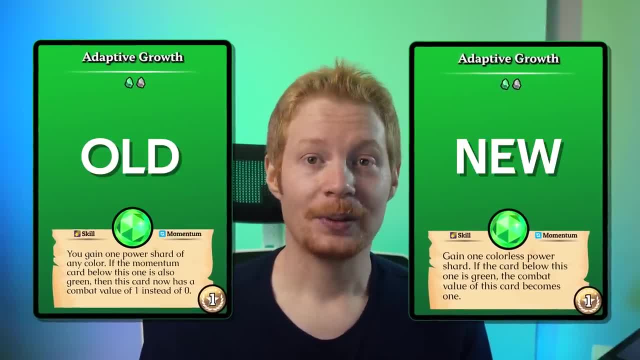 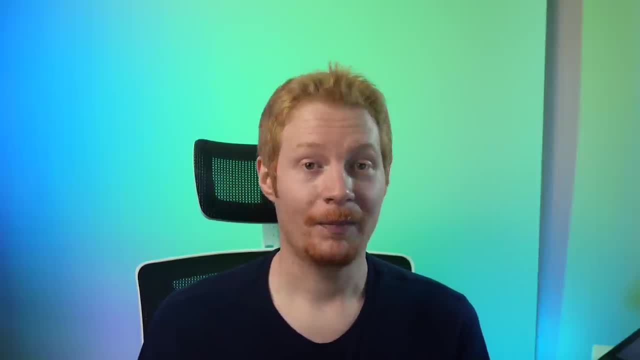 ten times better. This one sounds like a proper rule. Golden rule number three: If it can be said in fewer words, say it in words. Cards are the most interactive component of a game. They are the driving force that make your game work. They need to be engineered for readability at a glance while containing a ton. 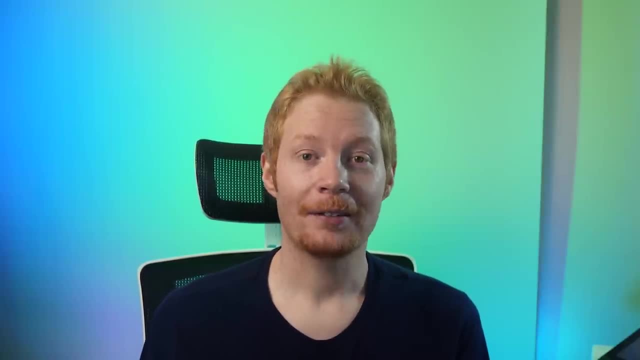 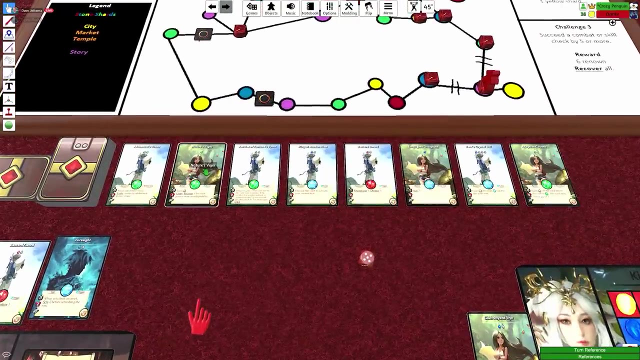 of information and still look cool as heck. No one wants to read a paragraph. Nobody got time for that. We have eight cards laid out in the middle of our table. If each card is filled with text, that's practically a book. Here's an example from our previous version of our game, where we went a 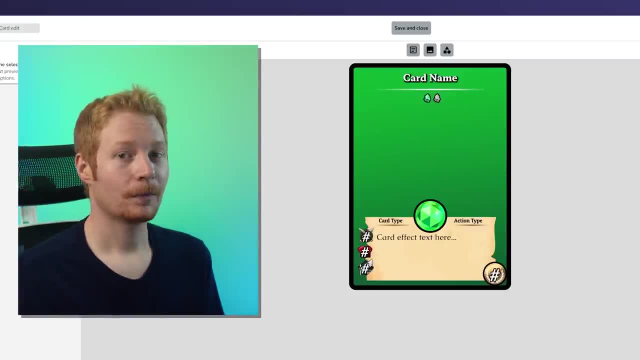 little too overboard. Back to our example card. We've brainstormed a bit and tried out a handful of different layouts and settled on this one for now. We understand that text should be said in as few words as possible, but we can take this a step further with golden rule number four. What do each 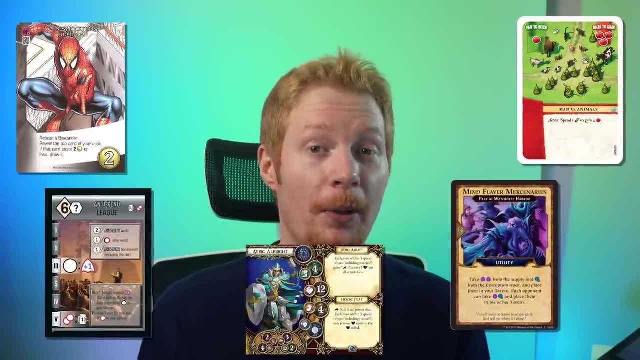 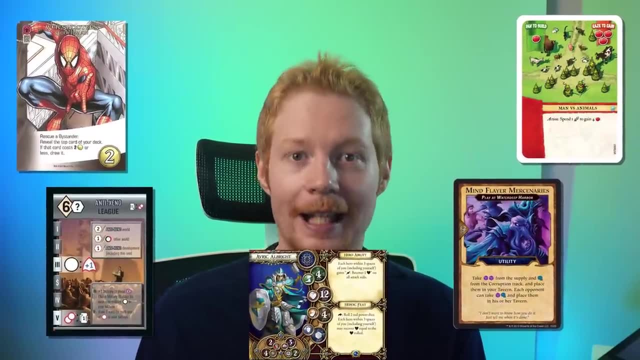 of these cards have in common? We're still looking at the effect text. What do you notice? It's something that wasn't in our previous example. I've always taken it for granted. I've been playing games long enough that it's become a second language at this point, something I can read. 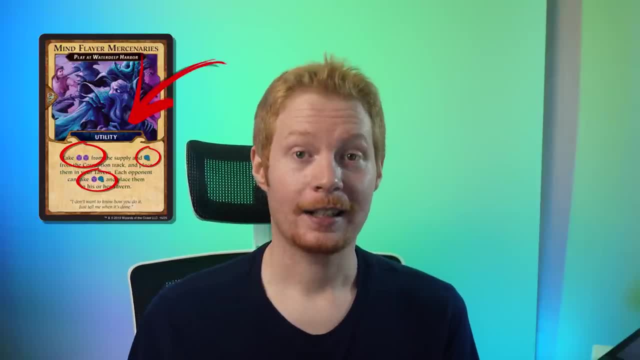 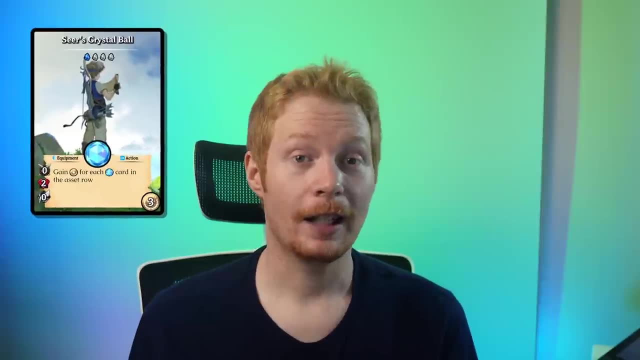 The thing I'm trying to draw your attention to is the iconography on the effect text, the symbols. In our previous version of our game, we had a couple of different ways to put this golden rule in. The first is shown here, like the other examples I was just showing you, but also the same. but. 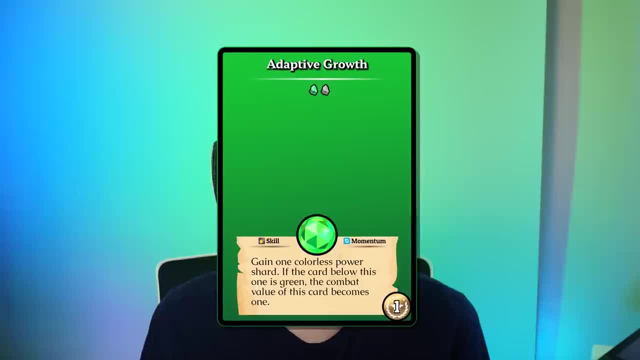 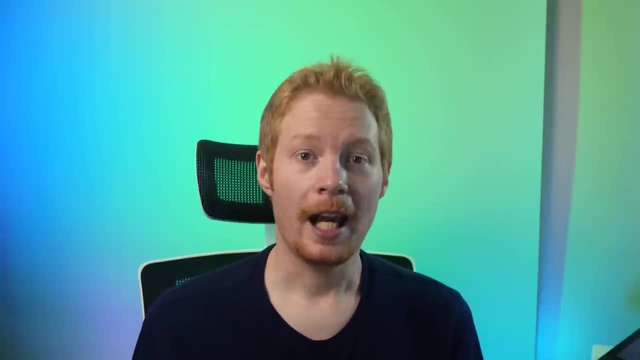 different with this card. Our example from the previous golden rule looked like this, and we leveled it up by saying things in fewer words, but we can take it a step further. This card reads: gain one power shard of any color If the card below this one is green. 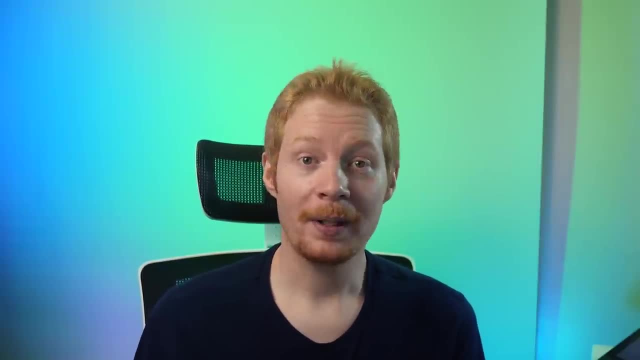 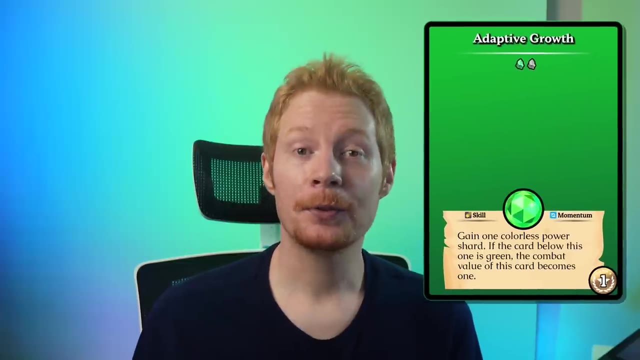 the combat value of this card becomes one. It's shorter than before, but the phrases gain one power shard and increase your combat value show up across many cards in our game. So we put golden rule number four in our game and we're going to show you how to do that. 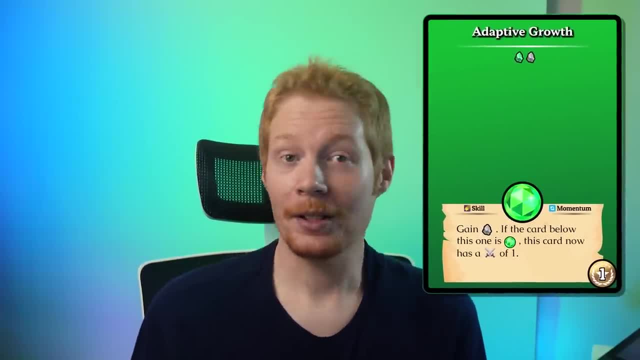 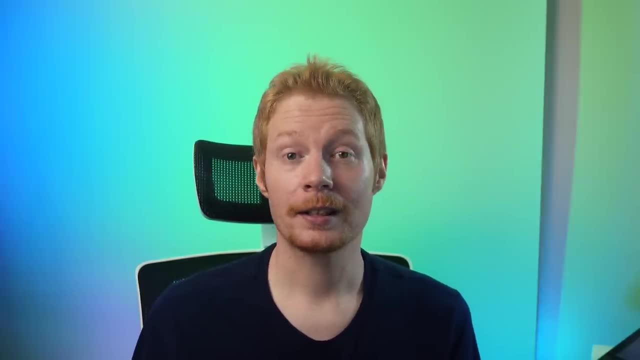 The golden rule is going to affect changing it to look like this. Your game probably also has recurring phrases or mechanics that pop up across multiple cards. This rule is very simple and it levels up your design just as much as the previous. Just make symbols. Golden rule number three was: 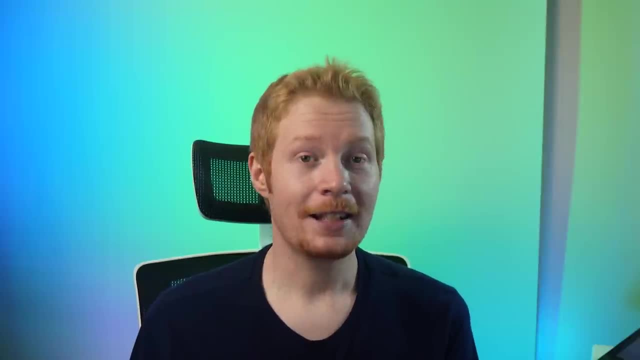 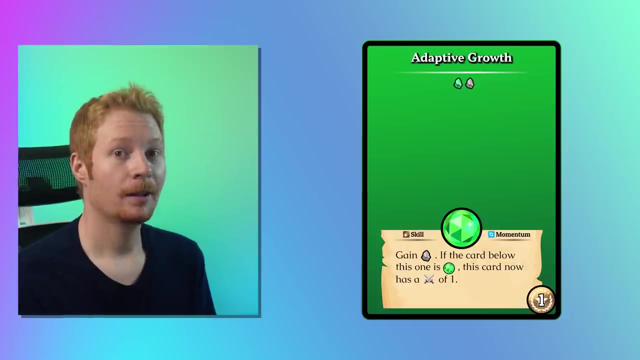 if it can be said in fewer words, say it in fewer words. The next is an extension of that Golden rule. number four: If it's said repeatedly, say it in symbols. So here we have what was once a blank card putting everything that we've learned into practice, but it's missing one important piece of. 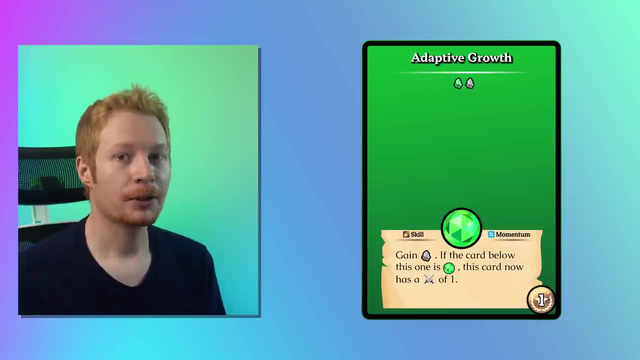 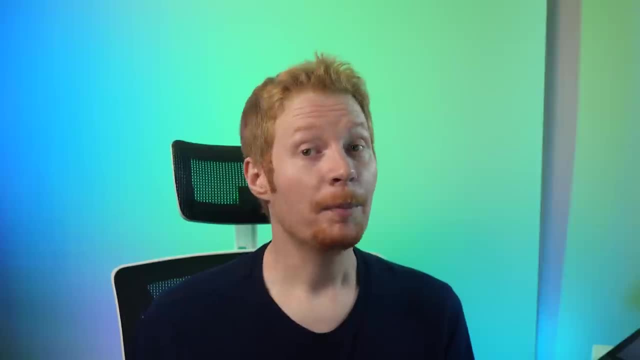 the puzzle All the way. at the top of the card we have a little bit of a rule that we can use to change the design of your visual hierarchy. family tree or compelling story was arguably the most important part of every card's design And it's the easiest one to guess. But before we jump, 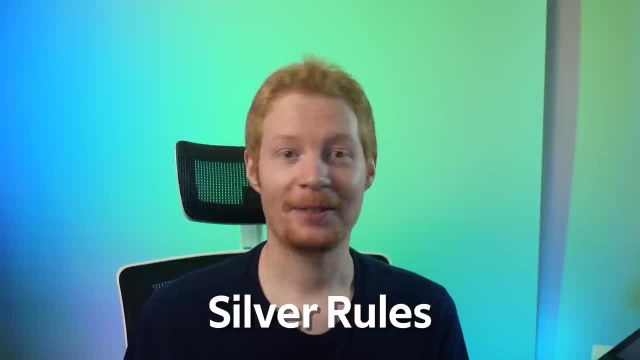 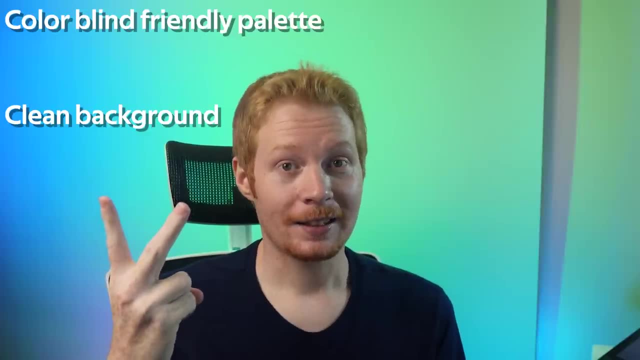 into the final golden rule, a couple of honorable mentions. Silver rules, if you will Consider colors that work better for those who have colorblindness. Choosing the right background can help a ton when reading text. Same with the right font, And keep the rules on the cards, not in the 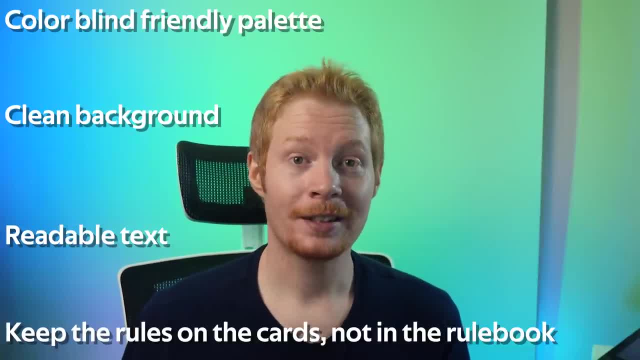 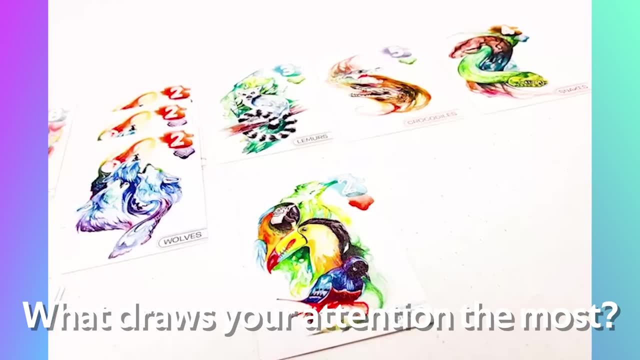 rulebook. If you find yourself adding rules that relate to a small number of cards, find a way to fit it on the cards or axe those cards. What makes a card look good? What draws your attention the most? I love each of these cards. 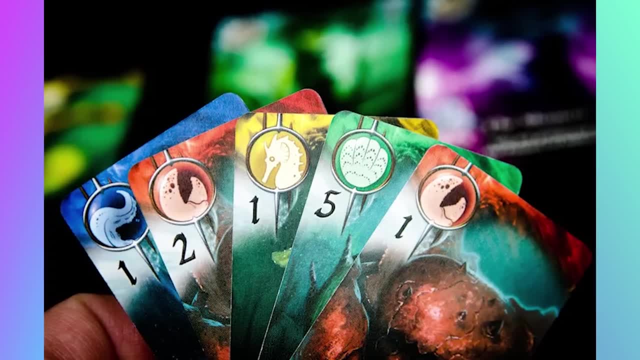 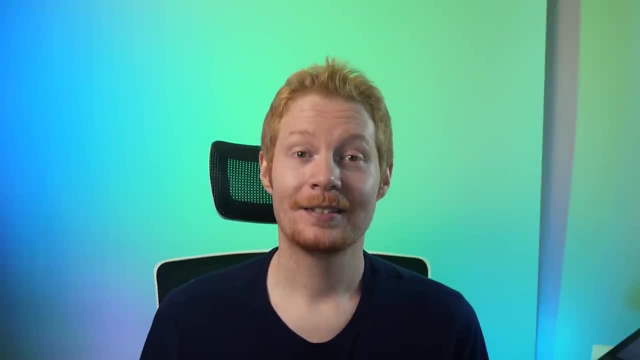 for the same reason. I wonder if you like them too. I think they're pretty, They look cool and I want to hold them in my hand. A compelling visual design is a big part of what makes your game awesome, And that extends to your cards. It's weird: Art doesn't contribute to the playability. 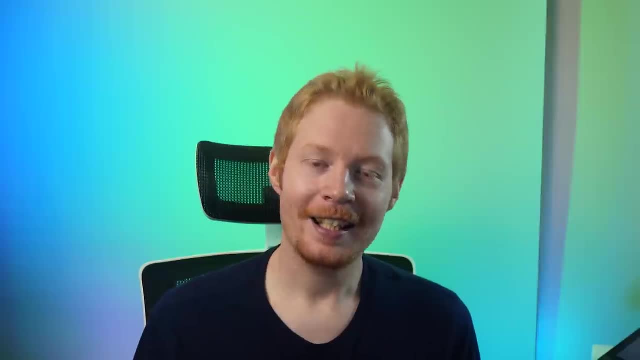 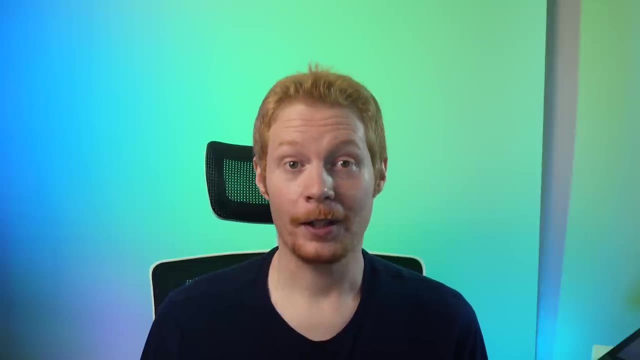 of your game at all right. It's just eye candy, And yet it takes up the majority of most cards. Art is what draws people in. It's what caused me to go out of my way to talk to the developers of the game And it's the reason I stopped in my tracks and asked Matt to tell me about his game. 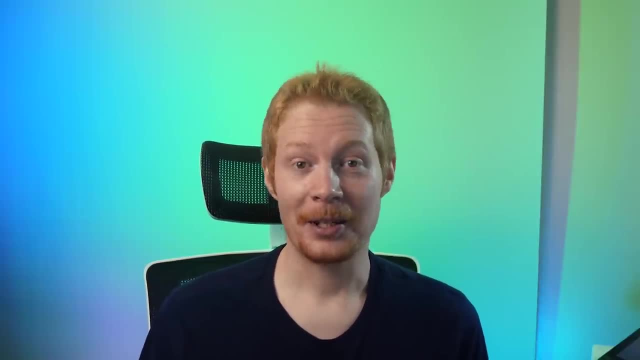 Flock Together. Ironically he has the same artist for Everdell and Farshore. But art is more than just being fancy or looking good. Art is the glue that holds all the other elements together. It creates a framing effect that draws your eye and reinforces the theme of your card. Golden rule: 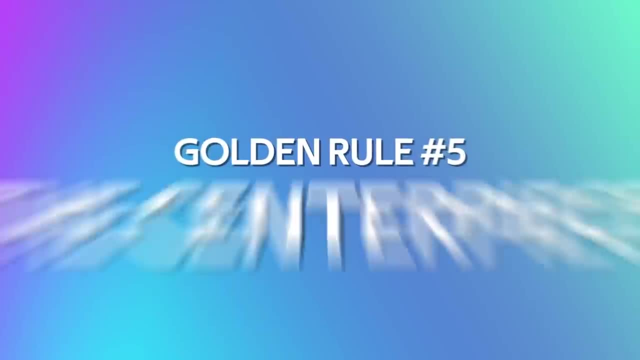 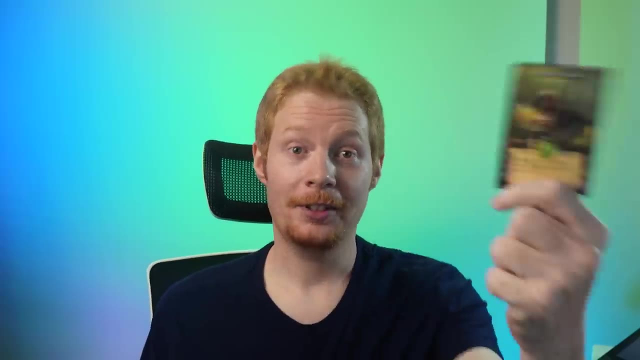 number five: Art is paramount. Or more accurately, make art the centerpiece without compromising function or design cohesion. But I like the phrase art is paramount better. So here's our finished card. that started blank. It still has a way to go, but it's more than enough to move on to the next step, If you want. 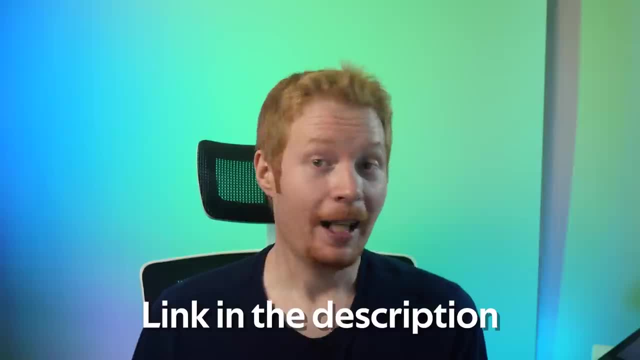 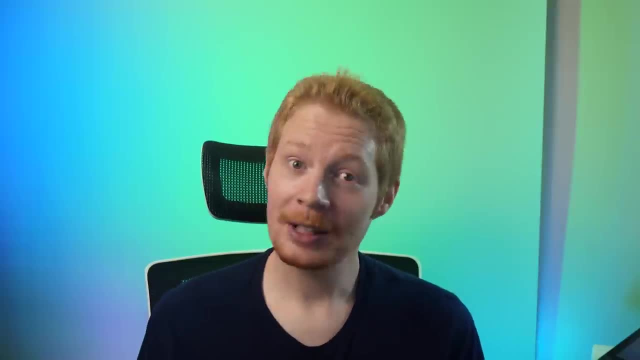 feedback on your card design. you can join us on the Tabletop Craft Discord And, if you'd like a jumpstart on your own project, I've provided links in the description with templates for the website that I showcase in this video, Dextrous. I was also going to provide templates for Photoshop and 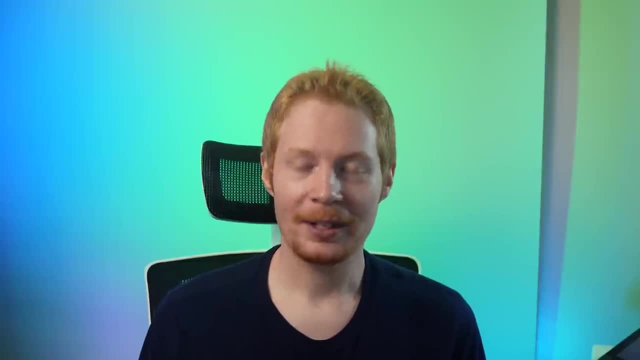 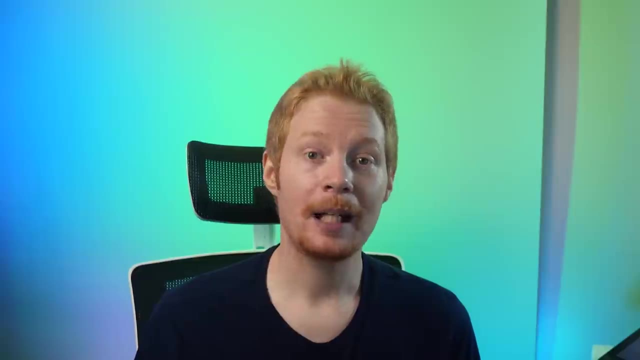 Canva, but then I would be setting you up to fail if I did that. Seriously, don't design your cards that way. I've got something better for you. Don't waste your time making changes to each card individually. Don't waste your time and money printing them out each time you make a change. 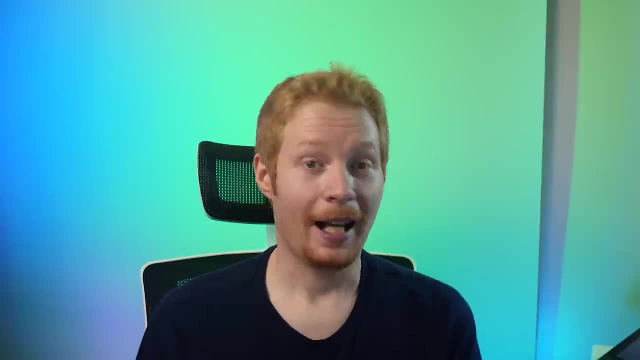 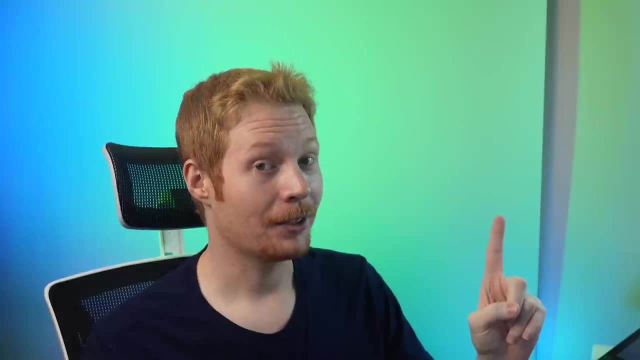 You're going to need to playtest, playtest and playtest some more, And I cover the best method to rapidly prototype and playtest your game in this video. I said I was serious and I meant it. This is a game changer. 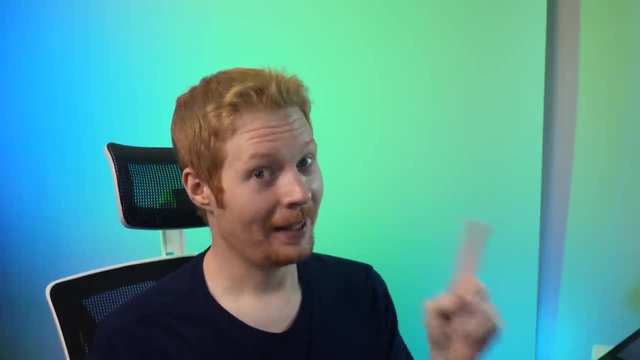 My name is Dave Geltema. I hope you learned something and I'll see you in that video.